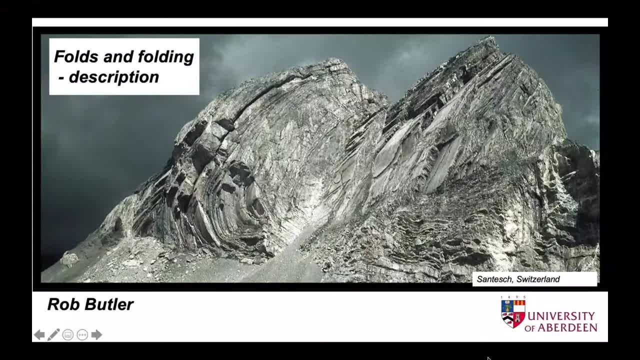 Folds are perhaps the most striking of all geological structures like this one on a peak in the Swiss Alps. Let's have a look at how to describe these folds and introduce the terms and how to apply them. Let's move away from the Swiss Alps to North Uist and 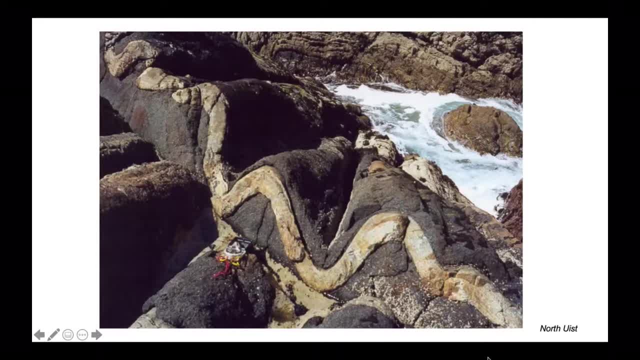 we can see this rather nice folded aplite layer within amphibolites. Let's use this to build some terminology So we can describe the structures as antiforms and sinforms. So antiform is the up fold, so an upward closing fold, and a sinform is a down fold or a downward. 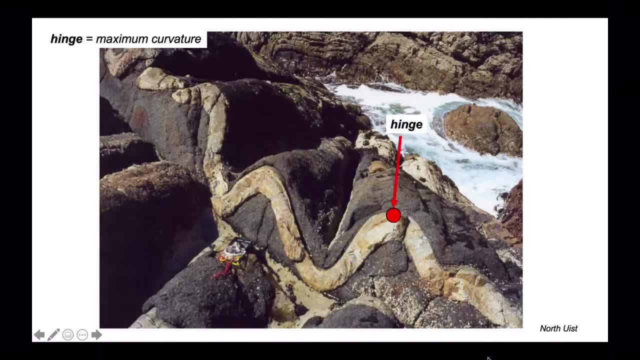 closing fold. So let's look at the geometry of these structures. We can identify a point of maximum curvature here, which is a hinge, and consequently the pieces on the side here are the limbs. Each fold has its own structure, Each fold has its own hinge on this layer. Let's just consider the three antiforms that. 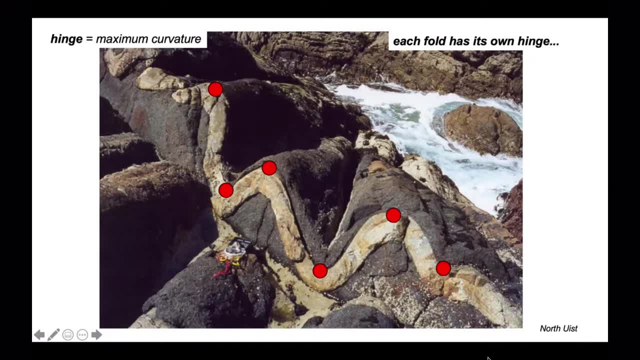 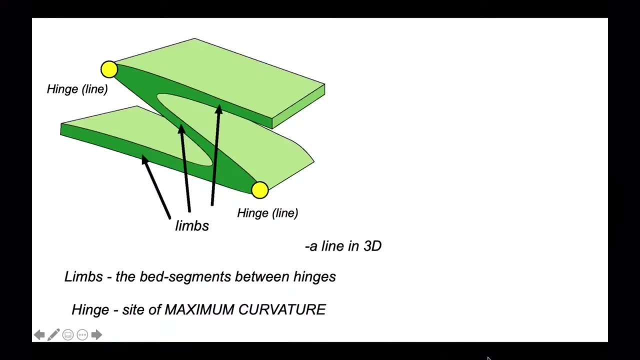 we've picked out on the photograph And we can see that the hinges are lines in 3D space trending off down towards the water like this. So the hinge lines are plunging down away from our viewpoint. So hinges are the sites of maximum curvature. The limbs are the pieces in between that are 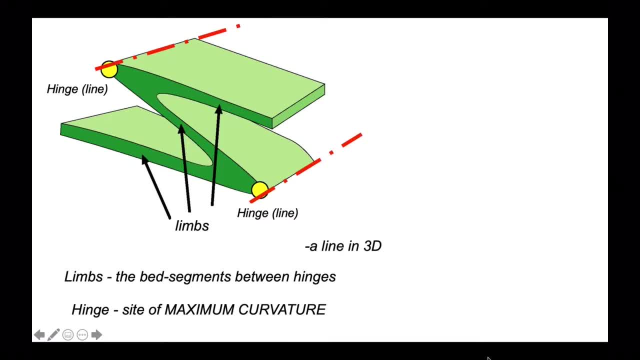 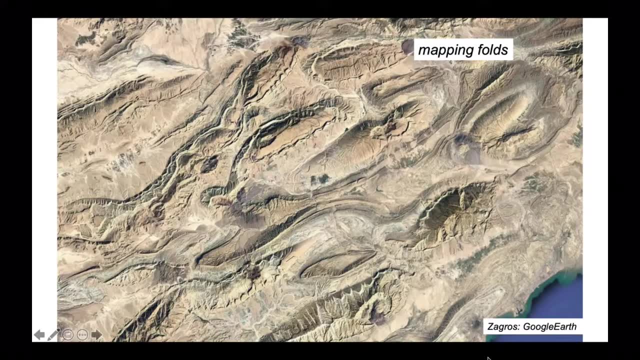 less curved And the hinges are lines in 3D space. Let's see if we can recognise some structures now here on the satellite image for part of the Zagros fold belt in Iran. Let's see if we can map some things out. So we're going to go and zoom in on some of this. 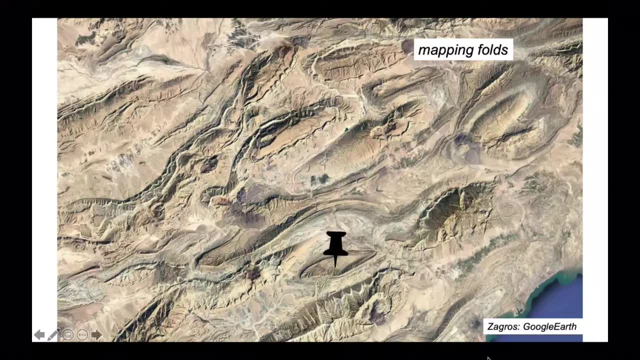 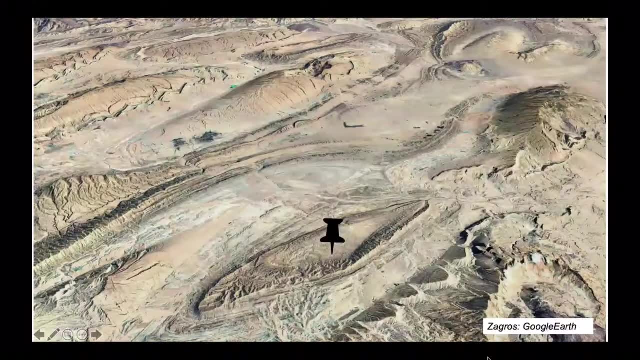 place And we're going to zoom in here where the pin is. So keep an eye on the pin In we go. We can see some really dramatic structures here And let's see if we can build a transect across this, starting down here on the right. 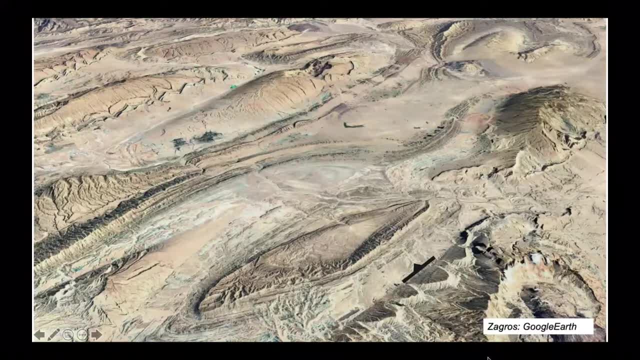 So, using this symbol, this shows the trend of bedding. You can see it in the landscape. So the length of that bar is the strike And the triangle on the side denotes the direction of dip. And as we go further across we can see the rocks retain the same strike and they're still. 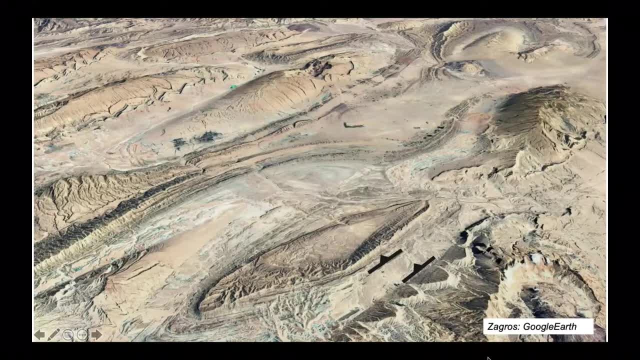 dipping into the ground towards their left. And if we go to the other side over here, we can see the opposite occurs And that's the same strike that we've seen in the other side. So we can see the opposite occurs where the dip direction is down to the right. 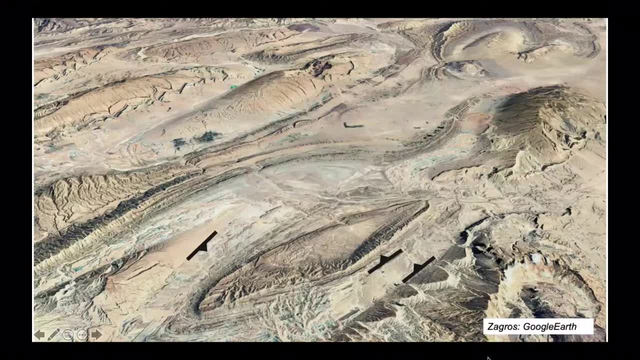 The neat thing about this image is we can trace some of the layers around the structure like this. So, looking into a fold, the beds on either side of the fold dip down towards each other, So we're dealing with a sin form And there is the hinge line running through the landscape. 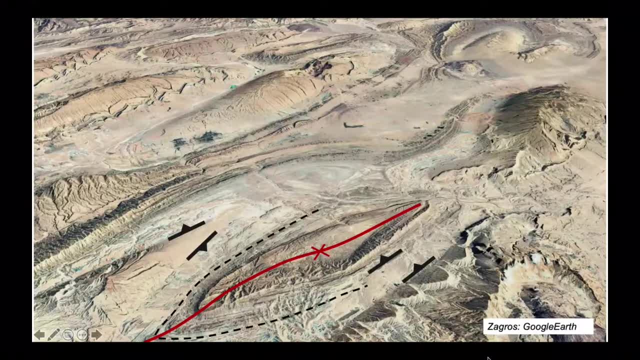 So let's continue to the left, And we can see here that the dips dip away from our previously most left hand symbol, And again we can trace some layering around the structure. So we've found another fold and it's an antiform like this: 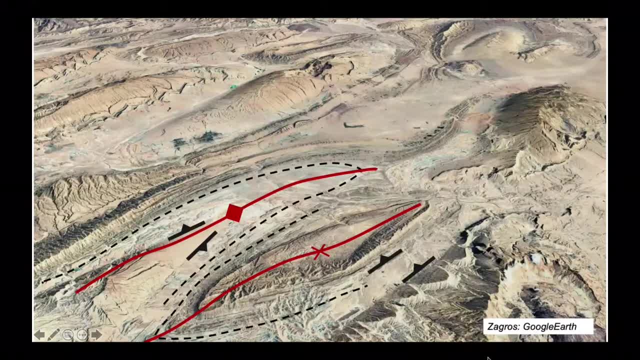 Let's see if we can spot another antiform. Well, there's one that re-traumatic big whale back structure And if you look really carefully, between the two and forms that we've got there now, there's a sin form that runs through here. 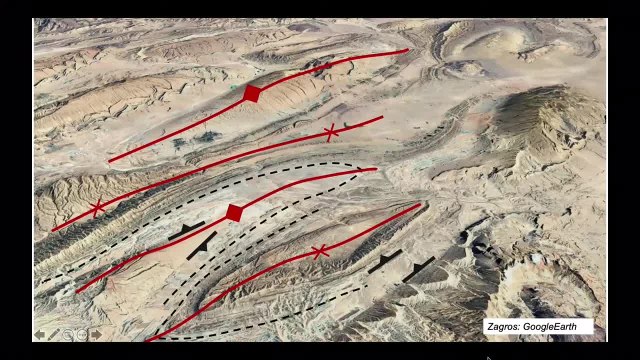 So here are some folds in the landscape. Thank you, We're going to zoom out. now let's put some locators. we've put our pin back in the sin form and we can put a flag on that far anti-form over there and let's look down on them from. 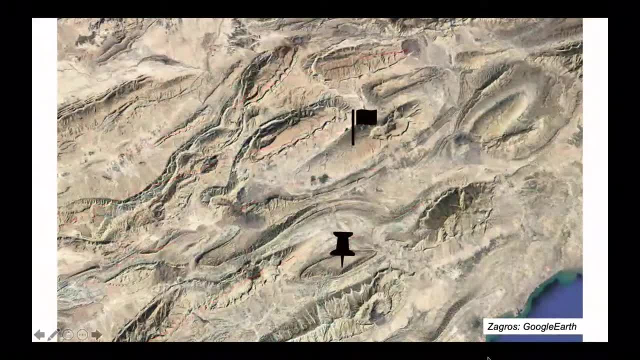 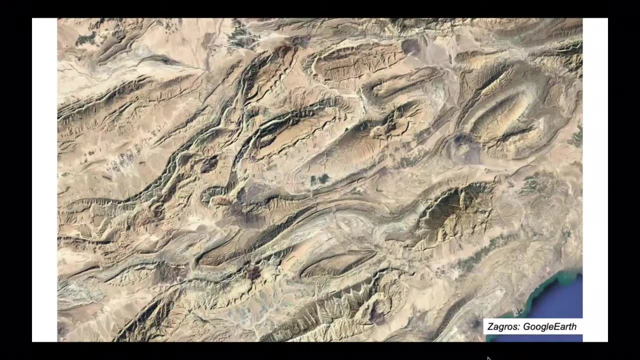 above again. Here we go. so those are those structures. let's just take those symbols away and put on the structures we've interpreted. there we go. So we've got two sin forms, two anti-forms in the landscape and we can use this approach. 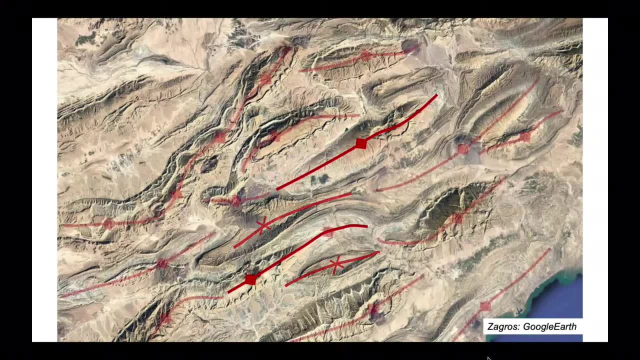 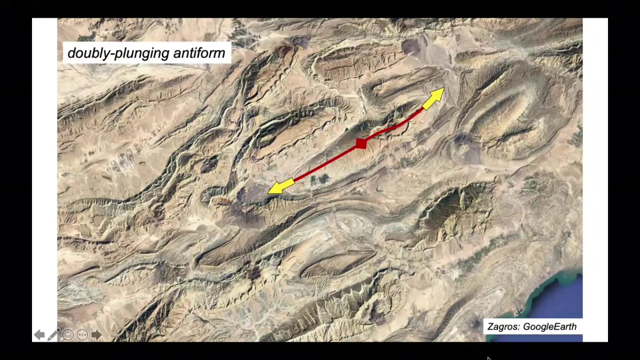 to map out others. All we've done is pick out the anti-forms for clarity, the sin forms we've mixed away. So let's zoom back into this structure here again so we can see that the hinge of this anti-form dives off towards both ends of the structure. 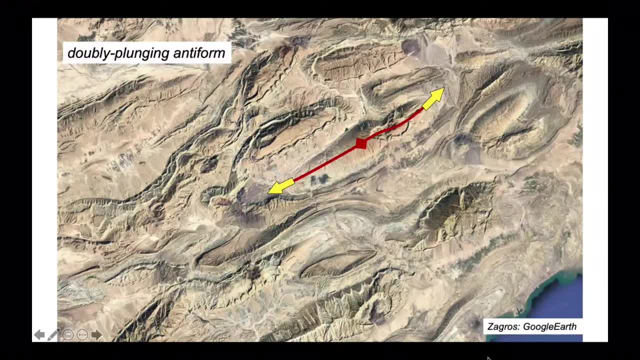 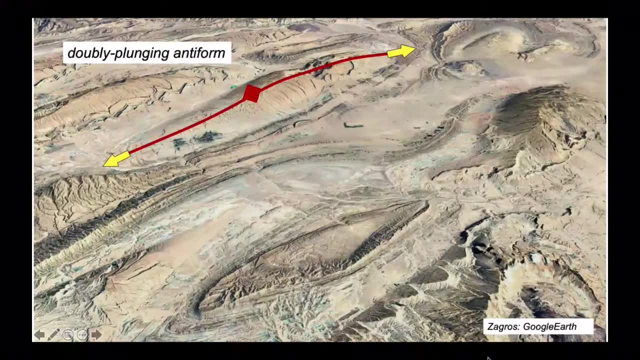 It's a doubly plunging structure. perhaps that's clearer. if we zoom in, There we go, we can see the hinge line of the fold diving to both ends, so the overall structure looks like a large whaleback. Well, let's pop back out again. we'll put a flag on this structure. here it is, that's. 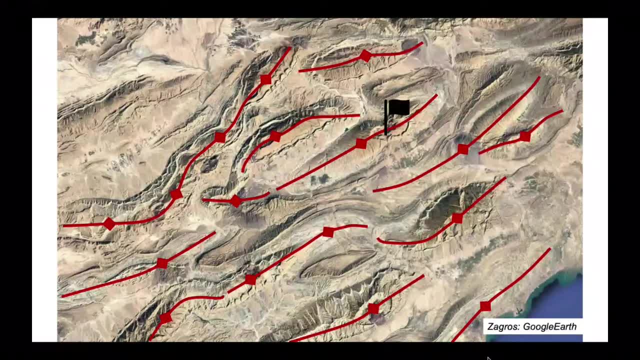 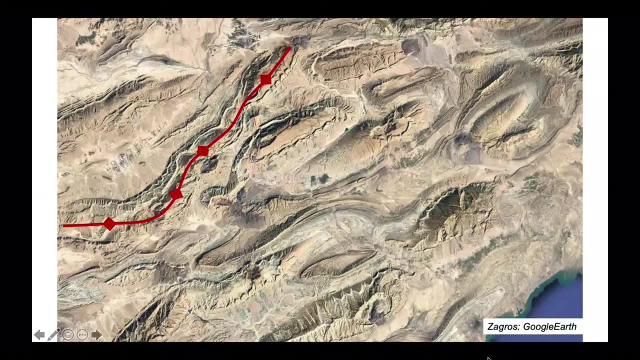 the one we've been looking at. let's look at another one in here, This one in here. look how irregular the trend of the hinge line is as it runs through the landscape and we can recognise along the hinge line. the hinge line is variable. 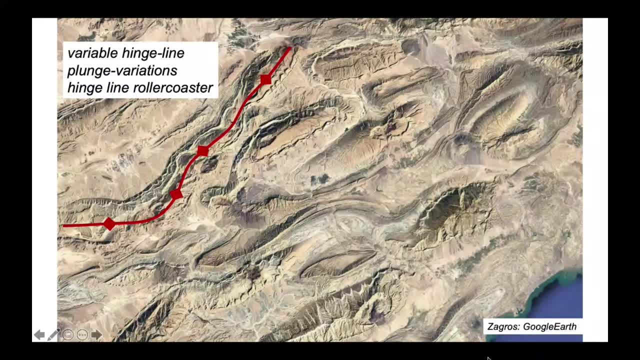 and there are plunge variations along it and the hinge line itself roller coasters along like this. so the arrows denote the ups and downs, pointing down the plunge directions of this hinge line. So the hinge lines don't have to be straight lines, they can roller coaster along their 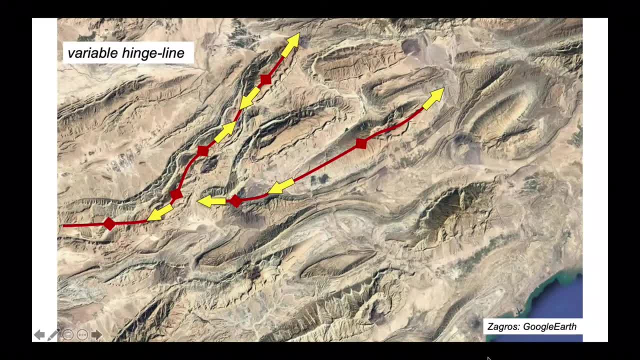 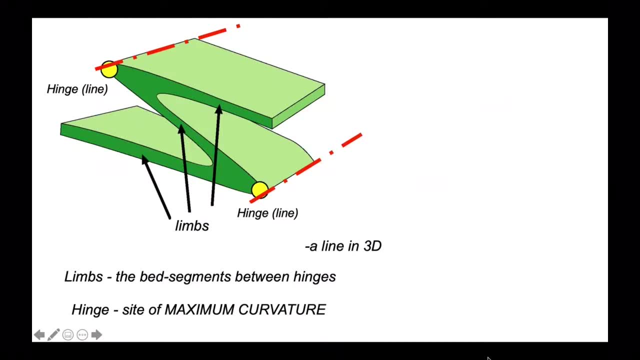 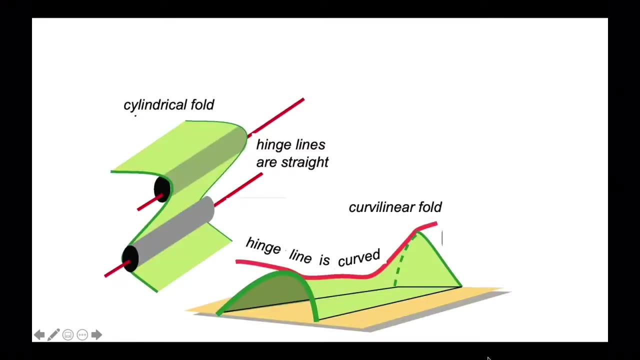 length and we've seen that in these both examples. So, coming back to our idealised cartoons, we've looked and defined hinge lines using this diagram, but the range of shapes can be more complicated. When hinge lines are straight, the fold is described as being cylindrical. if the hinge line is curved, like we've seen in some of those examples, then the fold is also cylindrical. So if the hinge line is curved, like we've seen in some of those examples, then the fold is also cylindrical. if the hinge line is curved, like we've seen in some of those examples, then the fold is also cylindurgical. if the hinge line is curved, then the fold is also cylindrical. if the hinge line is curved, like we've seen in some of those examples, then the fold is also cylindrical. if the hinge line is curved, then the fold is also. 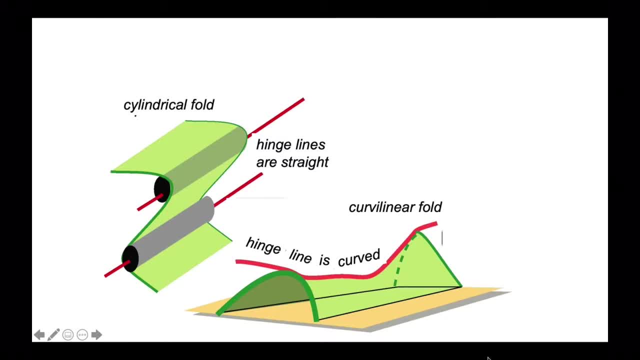 cylindrical, and so the cylinders can be curved too. If we have too many spaces on the autumn tree, aren't we going to have too many raises and variations in shape and size? So that's burst history. Let's take a look at some other examples of placeing force here, and colossal adding. 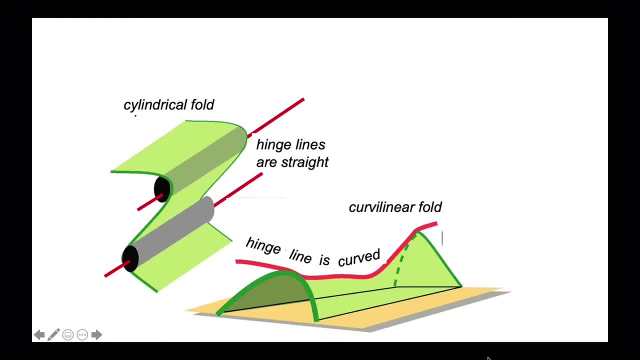 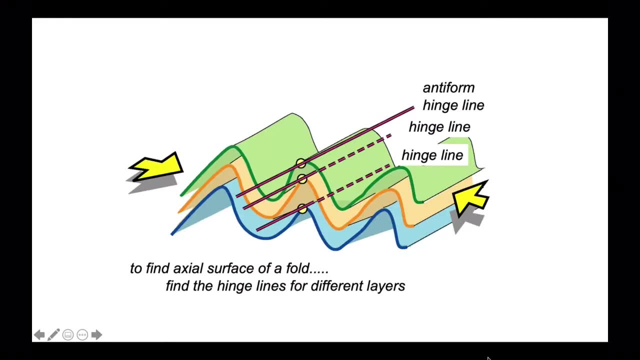 Gaussian waves. So here we've created this Honدي barrier on a flat surface. so I'll give a number of examples. Here we've just shown a scheme where we've drawn the lines as a dinosaur: Vogelbeiner. So if we put a series of layers through a fold, an individual fold structure- in this case the antiform- each layer has its own hinged line. 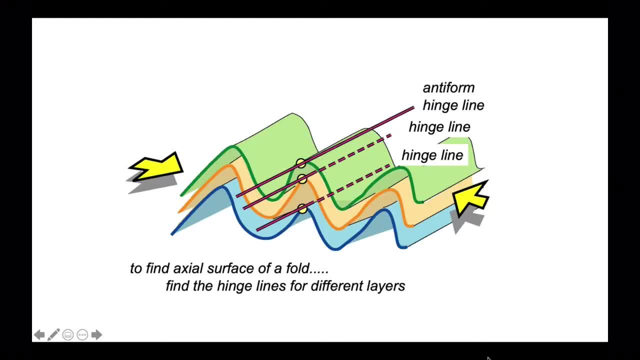 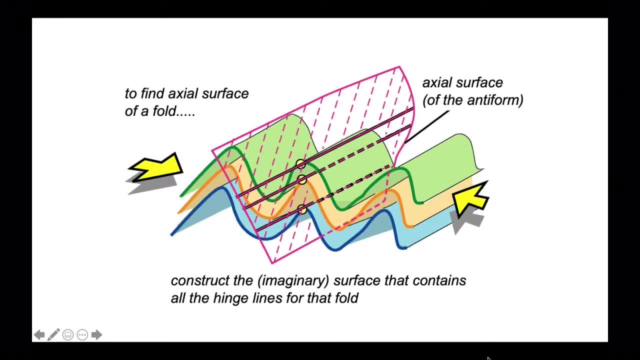 A really useful thing to think about is the imaginary plane that contains these hinged lines. It's called the fold axial surface. So it's an imaginary surface that contains all the hinged lines, that's for each layer but that particular fold. 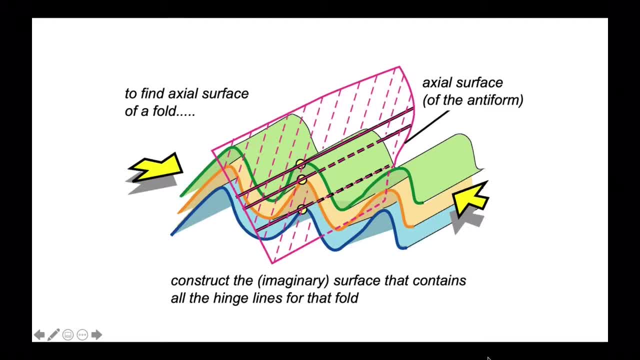 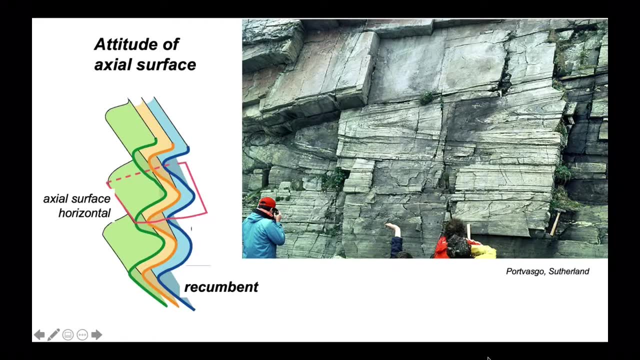 We can use the orientation of the axial surface now to provide more description of folds. So it's the attitude, that's the orientation of the axial surface. So here's an outcrop. It's a two dimensional representation, but obviously this is a three dimensional feature. 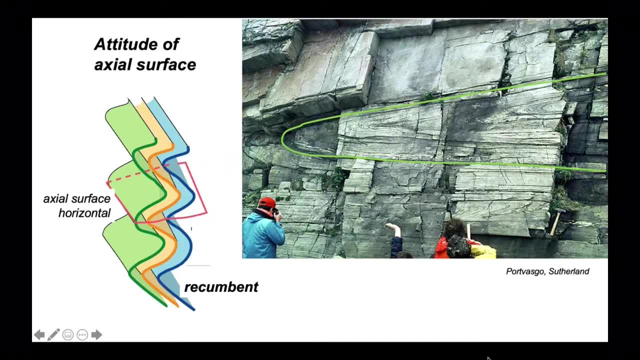 We can pick out some layering around this fold to define it and identify a series of points of hinges. The hinges will be diving into the screen If we join these up. it could look like this: It creates the trace of the axial surface on the outcrop and it's sub horizontal 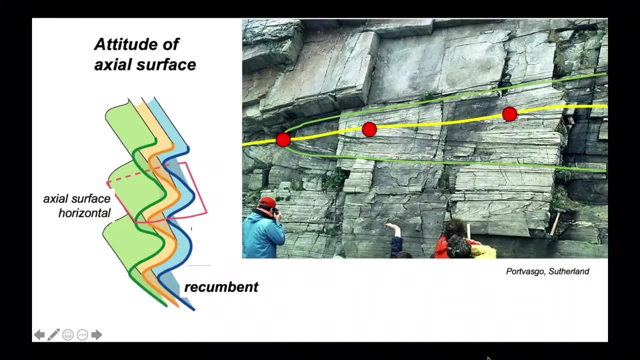 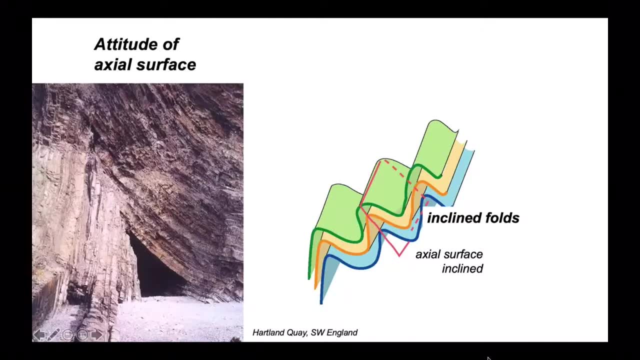 So we turn these types of structures recumbent. The axial surface is quasi horizontal. Let's have a look at another example here, And this time the axial surface will be inclined Again. we can recognise a series of hinge points, the hinges, the hinge lines diving into the cliff like that. 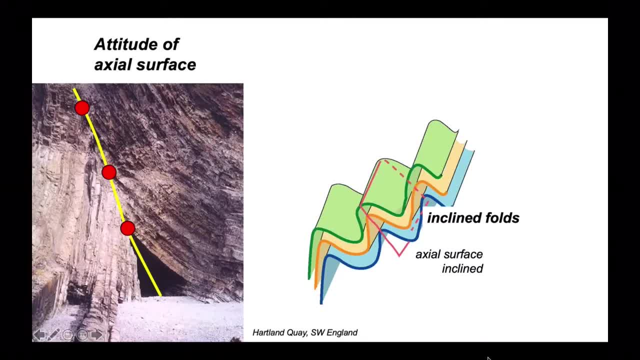 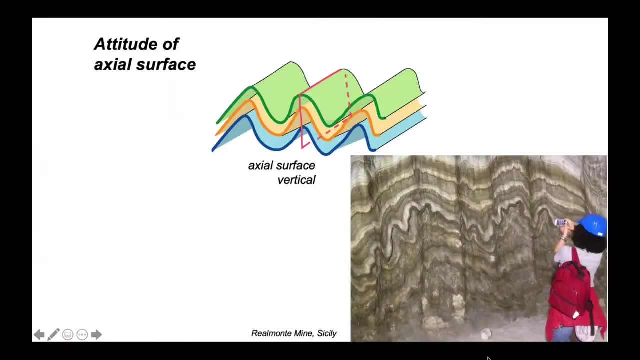 We can join them up. We can see the base of the axial surface on the cliff and it is inclined. So it's an inclined fold. Finally, here's an example from a mine in Sicily. We can see those folded layers, then trace on where the axial surfaces would be on the outcrop. 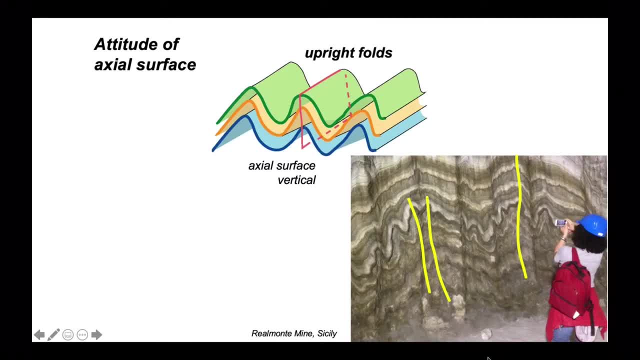 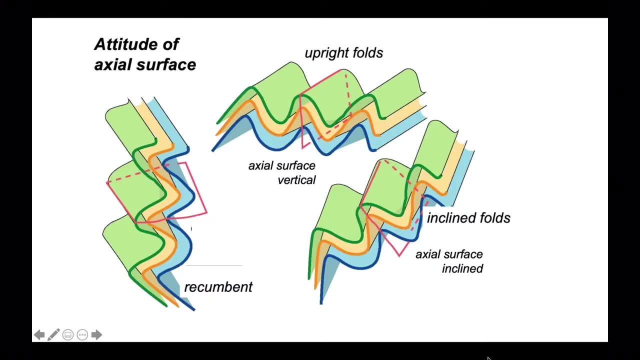 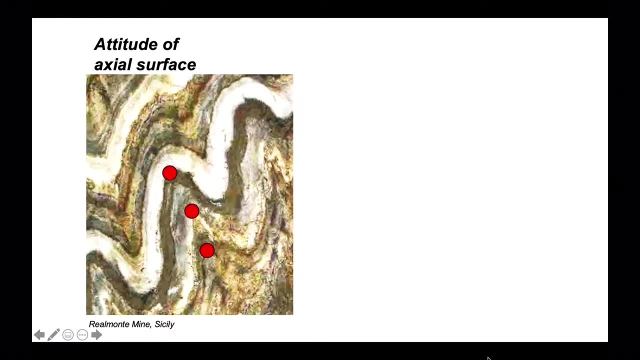 Here they go, and they're vertical, So these are upright folds. So a simple set of terminology to describe how the folds are arranged in 3D space Using the attitude of the axial surface. Let's come back to this now. We can recognise the hinge points, the hinges diving into the photograph, and recognise an inclined fold structure. 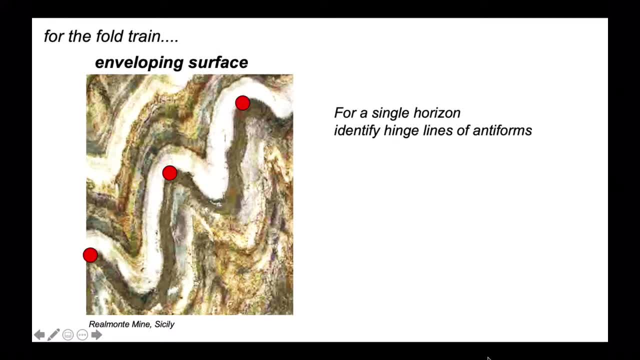 So now we're going to think about how an individual layer goes around a series of folds, And here we picked out three antiform hinges along the base of the white layer in the photograph. We can now create a so-called enveloping surface which would contain all these antiforms. 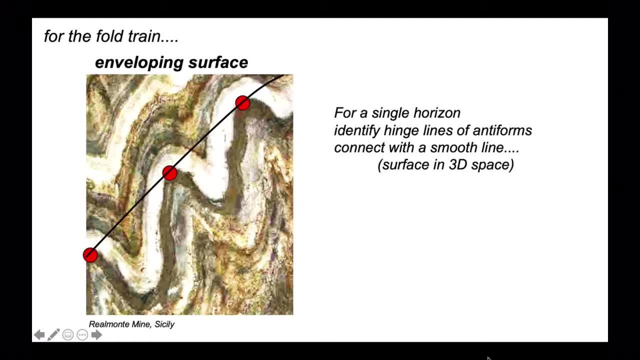 Here they go. So for a single horizon, we identify the hinge lines of the antiforms and connect them up with a smooth line which, in 3D, would be a surface going in and out of the outcrop. Now let's do the same for the sinform hinges of the same surface. 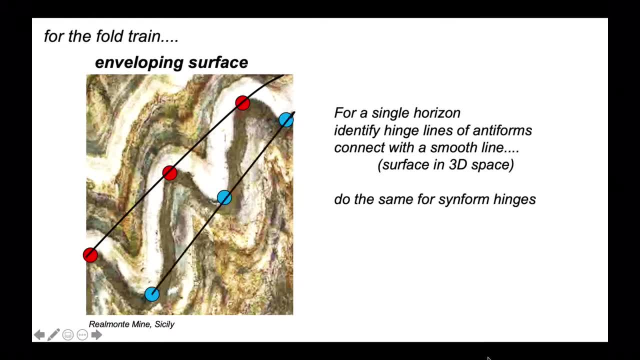 In other words the base of the white, and join those up, So that's the enveloping surface for the sinforms, And in doing so, the enveloping surfaces for the antiforms and sinforms will contain the entire extent of the base of the white layer. 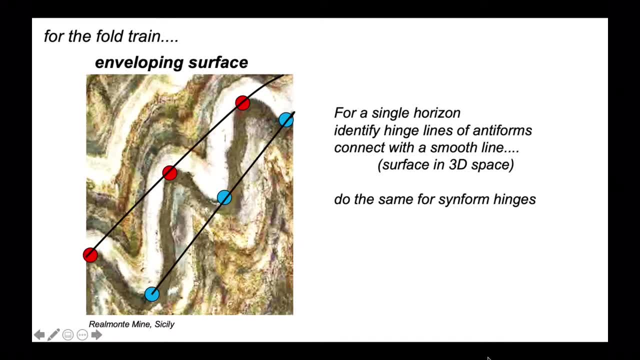 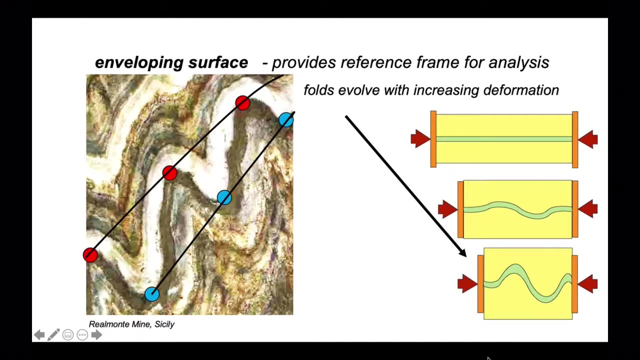 Hence the term enveloping surface. Now this provides a reference frame for structural analysis. Folds evolve with increasing deformation, and they evolve like this. The folds as they develop will increase their amplitude and reduce their wavelength. Now we can use the enveloping surfaces to provide a framework to measure amplitude. 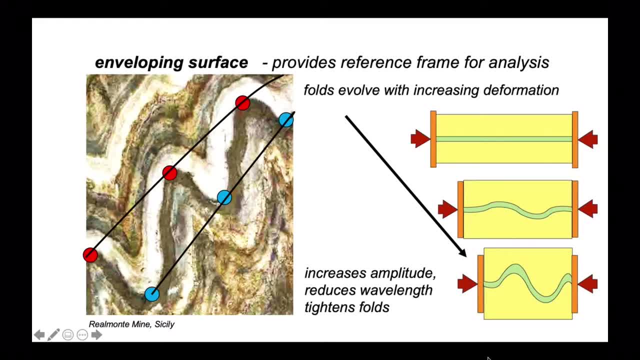 And wavelength. These are waveforms so they have the same terminology as any other waveform. There's the wavelength, And the separation between the enveloping surfaces is twice the amplitude. So we can make measurements now of fold structures and relate them to deformation intensity. 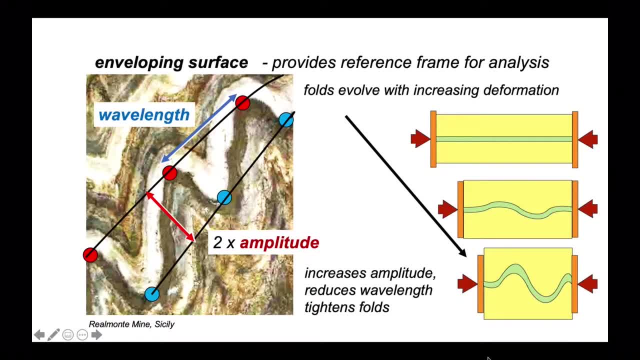 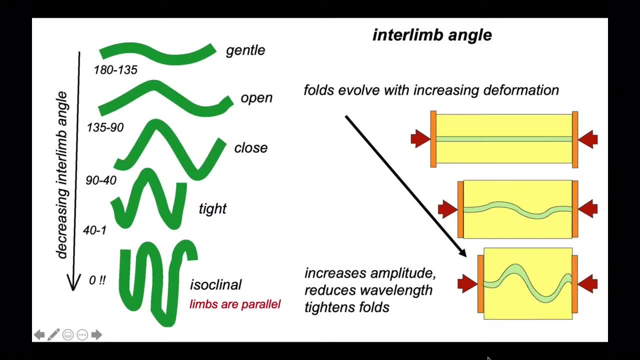 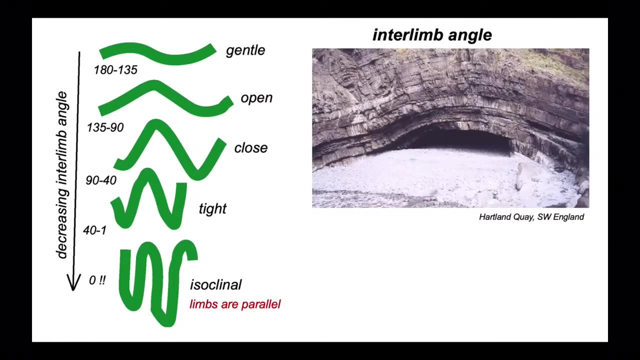 Qualitatively, we can use a description of fold tightness And this is the interlim angle, The angle of the layers between them And limbs. So let's look at some examples. Here's a gentle fold Where there's a very broad interlim angle. 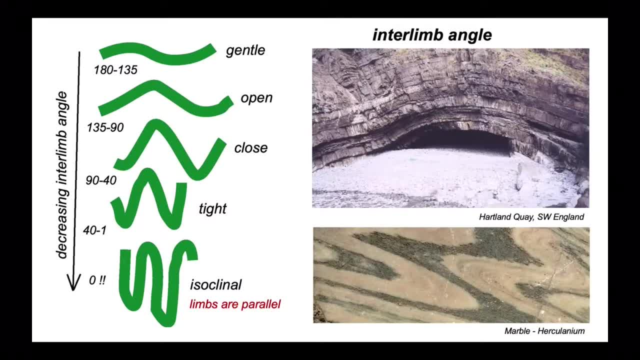 Here, in contrast, is a very tight fold, Not isoclinal. there's still a measurable interlim angle between them, But it's a set of tight folds. Now there's an important proviso here: We have to be careful to use the right cut or display through the folds. 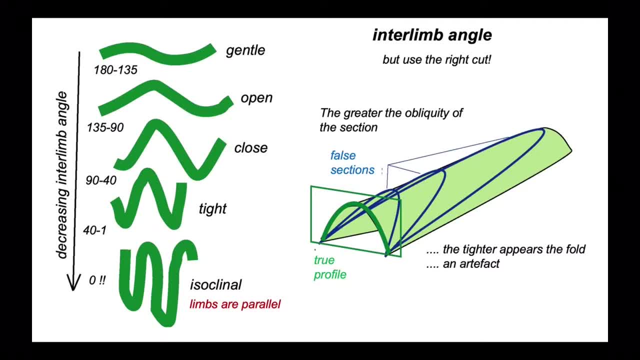 We need a true profile Which is perpendicular to the hinge. Oblique cuts give false sections And the folds will appear tighter than they really are. This is simply an artefact of the cut effect. So when measuring interlim angle or trying to get a view of interlim angle, 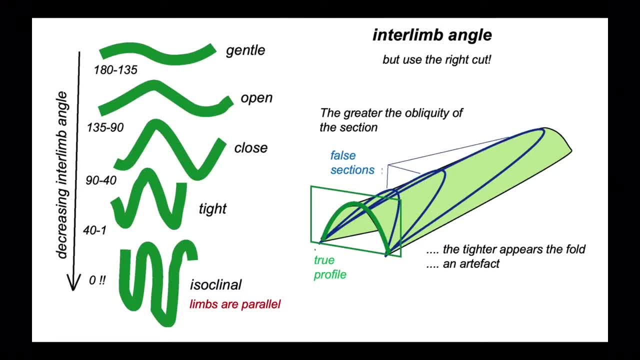 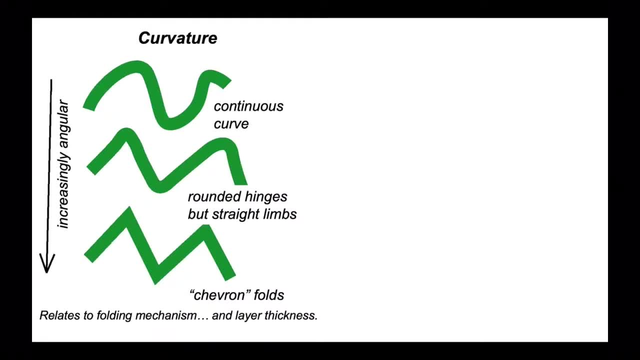 Always look down the hinge line. Okay, let's deal with some other aspects of fold shape. Layers in folds Can make various forms. They can be continuously curved, They can have very straight limbs And very sharp angular hinges, And they can have an intermediate case as well. 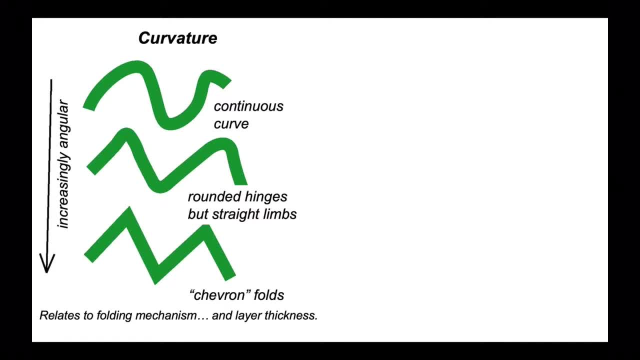 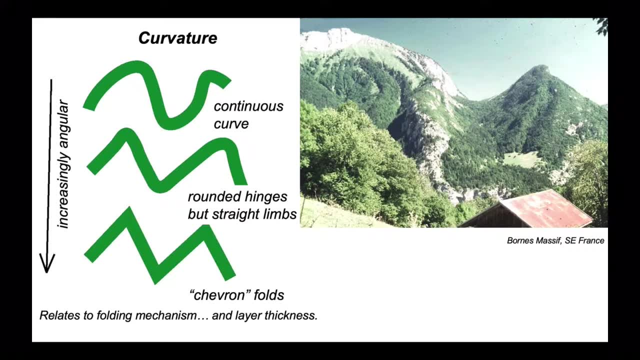 These shapes can be related to fold mechanisms, So making descriptions of them can be really useful. So here's an example of a fold in the French Alps, And we can recognise a continuously curving shape to this layer of limestone. So this is a continuously curved fold. 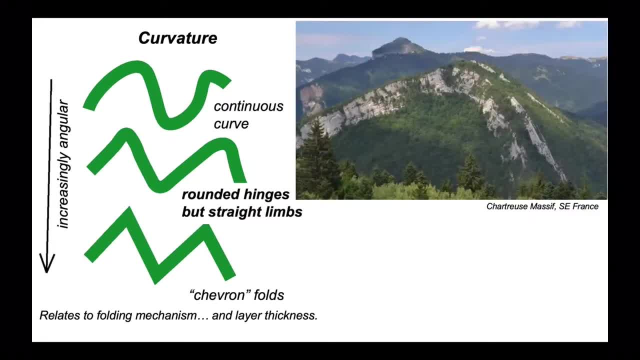 Here's another example. It's the same limestone units, actually in another part of the French Alps, But this is this intermediate case where we have definable long limbs And the area of curvature is restricted, But nevertheless, contrast those two cases with this one here. 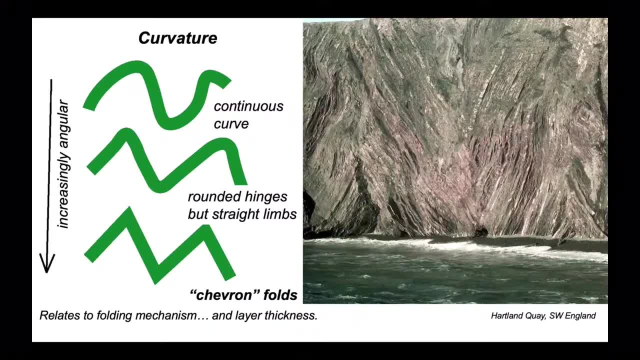 Which is some well layered sandstones and siltstones. Pick out some layering And we can see that the limbs are very straight. These structures are called chevron folds because of this shape. Okay, so many of these structures we've been looking at are pretty well organised. 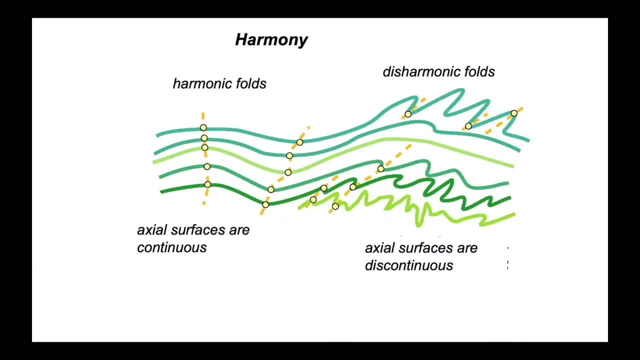 By organised I mean that the axial surfaces are continuous, So the shapes of the folds are harmonic. They don't have to be like this. But let's remind ourselves about what harmonic folding means. It simply means that we can trace the axial surface from layer to layer. 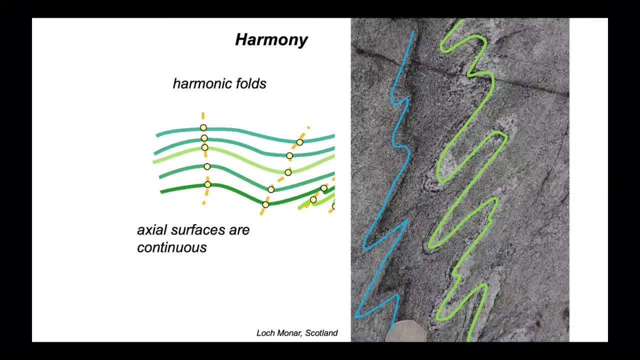 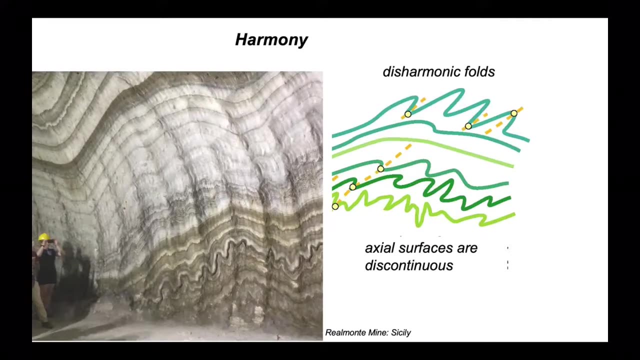 So if we pick these layers out here, we can trace axial surfaces continuously through, So each layer is folding in a directly comparable manner. But it doesn't have to be like this. The folds can behave disharmonically. So let's look at an example from this mine in Sicily. 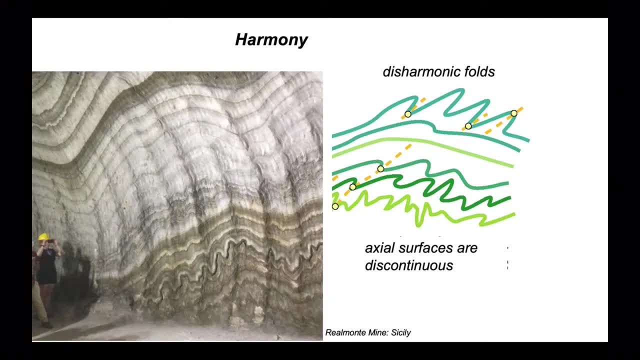 Incidentally, those big arcuate curves in the photograph are where the mining tool has carved the rock. They're not geological. Let's try and see through that and pick on this layer at the base And now pick on some other layers, So by the time we're at the top of the gallery, there are very few folds compared to the lower sections in here. 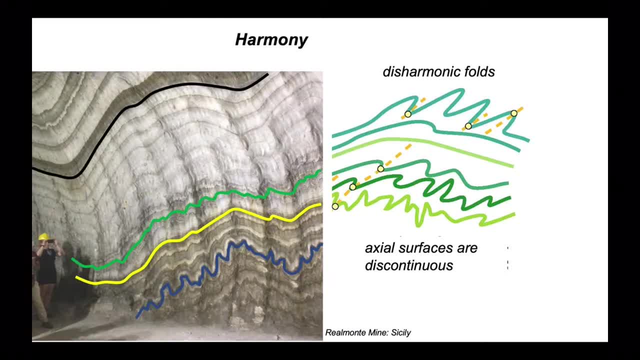 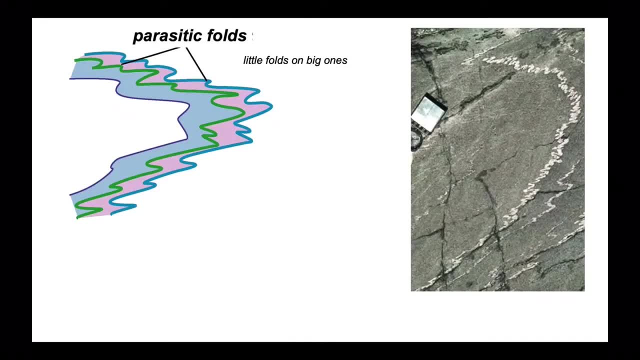 Consequently, the axial surfaces will be discontinuous. We're dealing with disharmonic folding. Folds don't all have to be the same size in an outcrop. So often you'll find little folds associated with larger scale folds. These little folds are described as being parasitic with respect to their relationship to the larger structure.